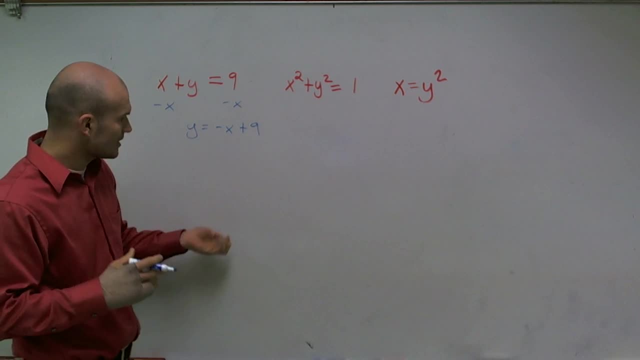 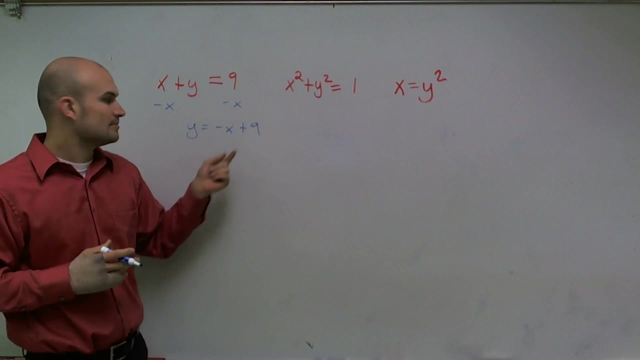 a negative x plus nine. What this tells me now is, for every term, for every x, I have a unique y, because if x equals, you know, 1, I'm just going to add 9 to it and I get a, you know 8.. But every single. 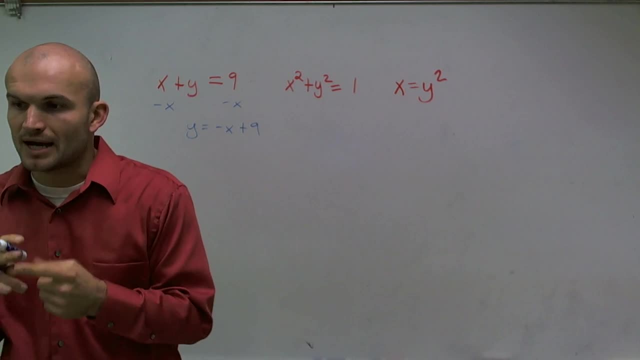 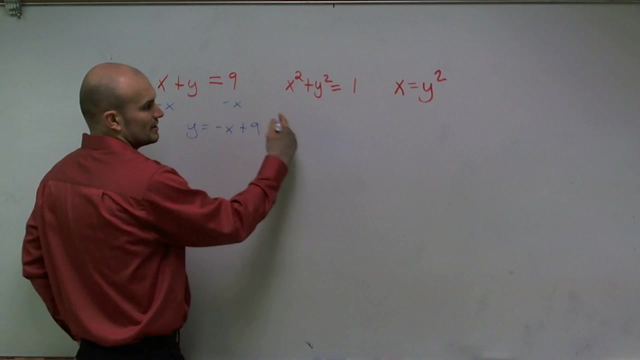 term is unique for my y. So since my output, I have unique terms for every input: x. this is a function of y in terms of x. If I look here, here what I'm going to solve for y, I subtract an x. 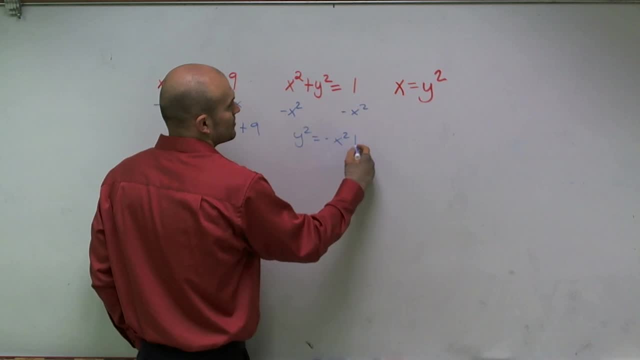 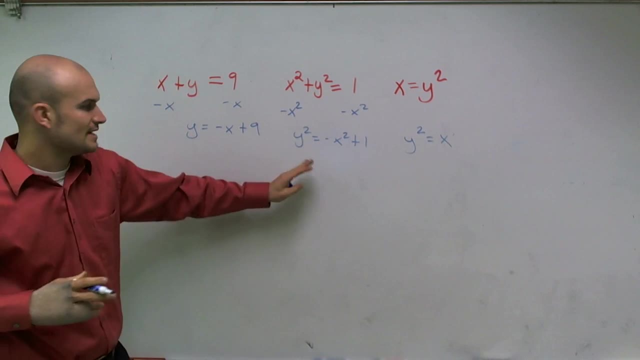 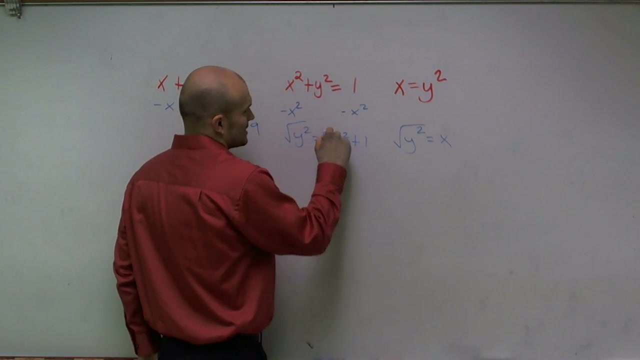 squared, I get y squared equals a negative x squared plus 1.. And here, if I just kind of switch those around, I get y squared equals x. Now, these two equations are different than these two because now to solve for y, what I have to do is take the square root on both sides And 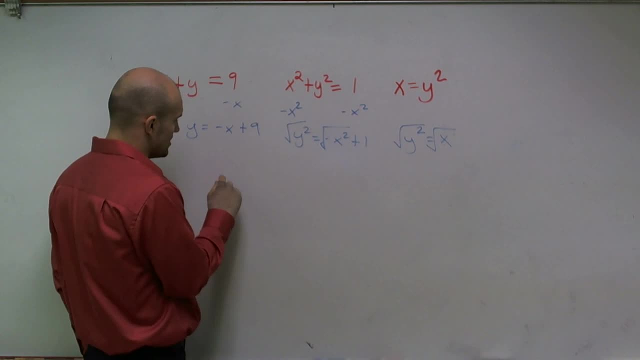 whenever you take the square root on both sides, remember the square root of a number. if I was just going to take the square root of 4, that could be 2, or the square root of 4 could also equal negative 2. Because, remember, 2 squared is, you know the opposite, Remember the square root. 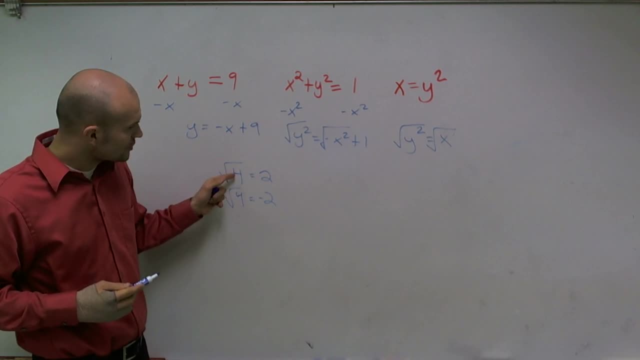 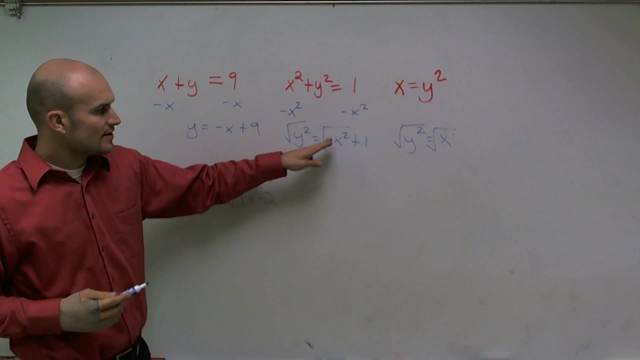 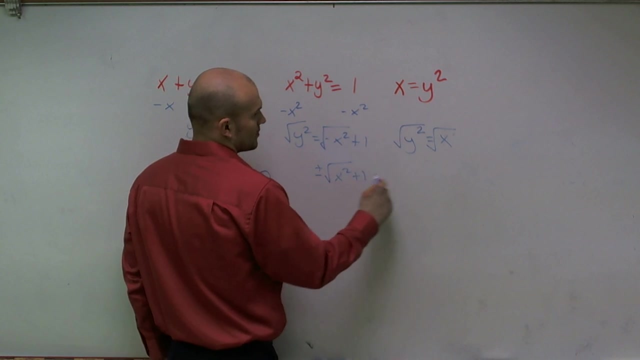 is what two numbers multiply to give you your, your radicand. So 2 squared equals 4, as well as negative, 2 squared equals 4.. So therefore, my answer here is actually going to be a plus and a minus: square root of x squared plus 1.. Here 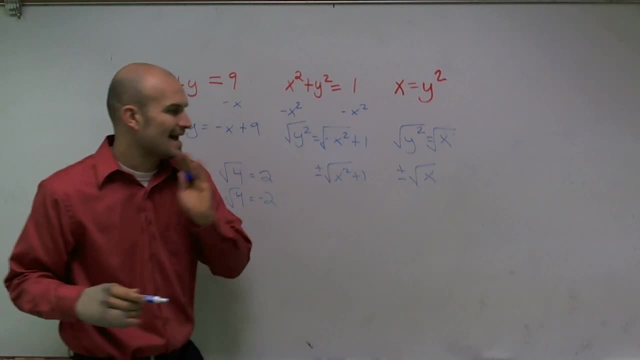 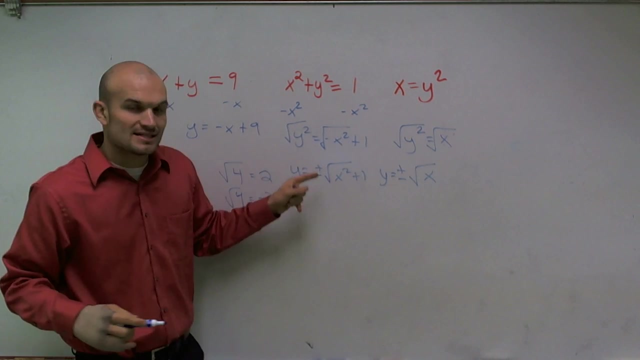 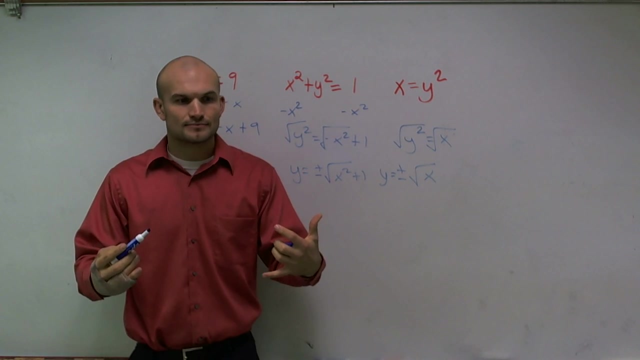 plus and a minus square root of x, Since I have two values for my x, for my y. see, I have a positive and an x Whenever I have two values. so it says: find which functions in terms of x. I'm sorry, find the function y in terms of x that are a. 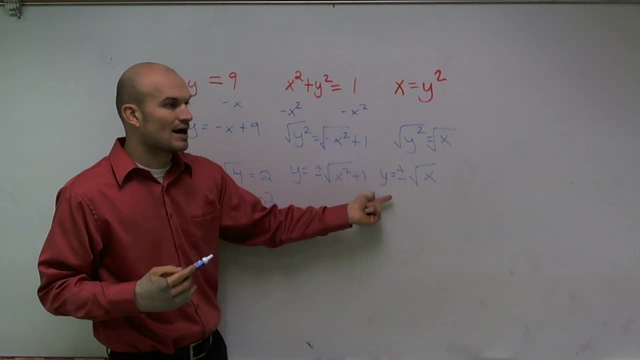 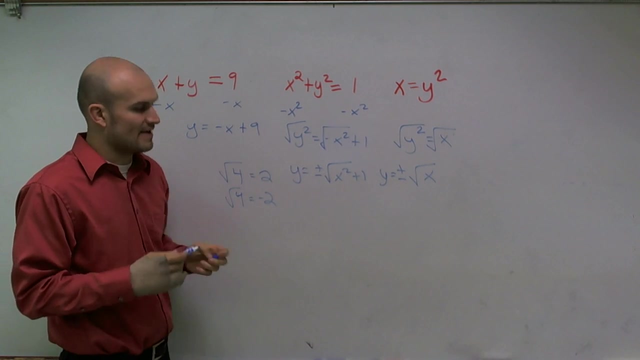 function Well, since my x's. I have two values for x for each y. this, these are not. you could not write these as a function of for y in terms of x. Here, however, every x value is going to. give me a unique y value. So therefore, that's why that one works.